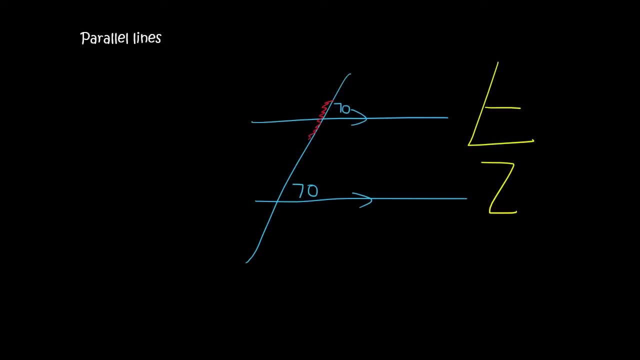 then if we look at this point over here, that is a straight line. so that means that this angle, these two angles, must be 180, which means that this one is 110. so then something interesting that happens is that this angle plus this angle will always add up to 180.. now, what shape are those ones forming? well, they forming. 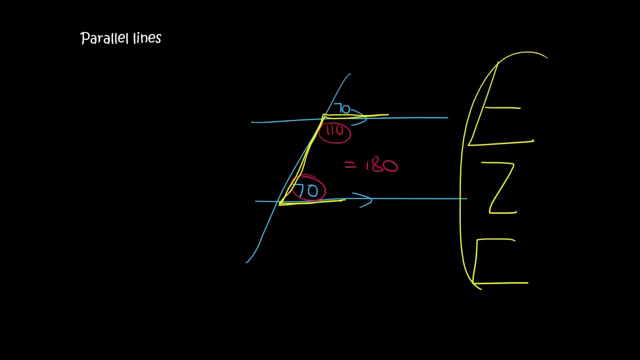 a u. so we've got something like that. so these are the types of shapes you need to look for. you need to look for a shape with an f, a shape with a u and a shape with a z or an n, and so always remember, when you're dealing with parallel lines, they are fun, okay? so if you can remember these three things, 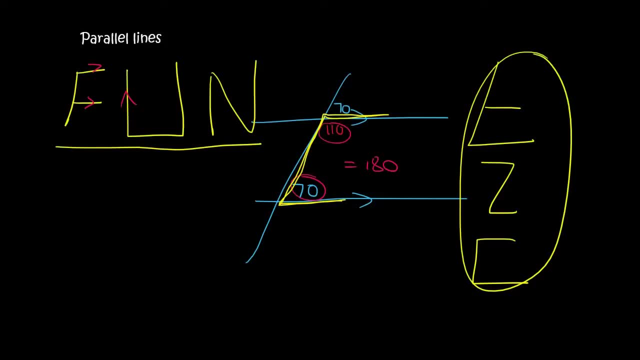 then you're good, so those lines over there would be parallel, those lines must be parallel, and those lines must be parallel. so then these angles are always equal. these two over here always add up to 180. they are not equal, but then these ones are always going to be equal to each other. the f: 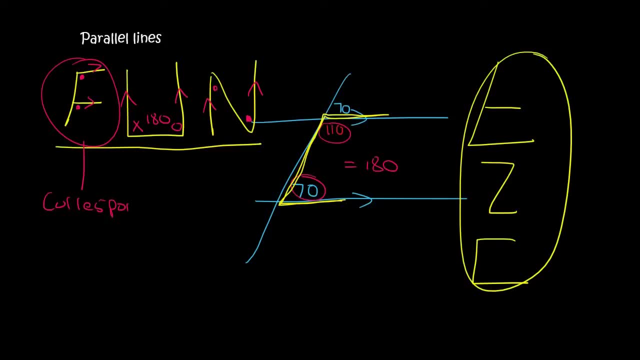 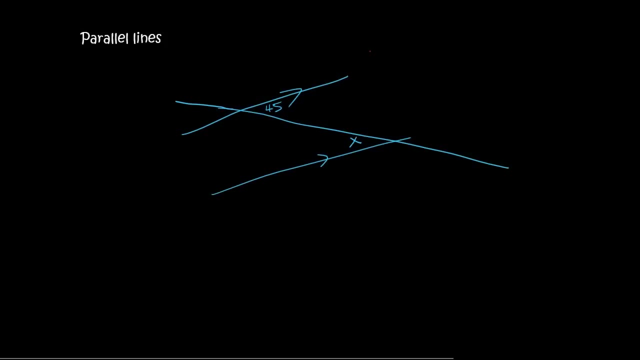 is called corresponding. in a test you can't say because of the f, but you can say that the f is called corresponding, the u is called co in teria and then the n or the z is called alternating. all right, so if i look at this diagram over here, i've got two parallel lines. 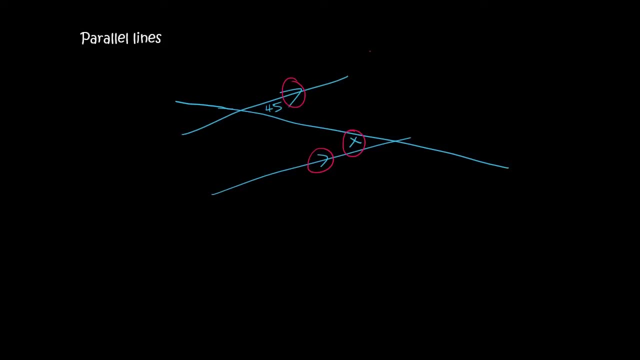 how do i know that? because of these arrows, i want to know what x is and i want to know whether it's the u, the f or the z or the n. the z and the n can be. the z can look like that, or it can be an n. 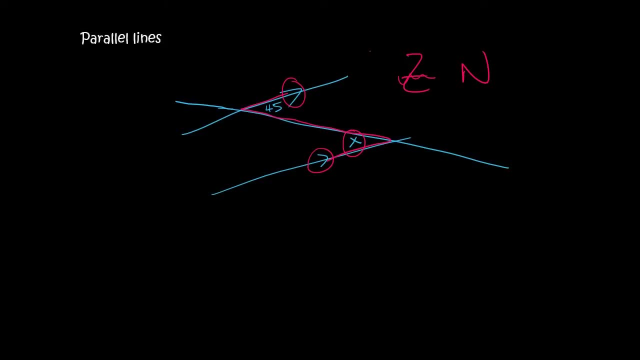 oh, we can see that it's a z, so we know that angles in a z are the same. so x would equal 45.. if i look at this one now, this angle is 120. so what will this one be? well, the shape that these two are forming is the u. and remember, oh, and these two should be parallel. if you have a u, then they're. 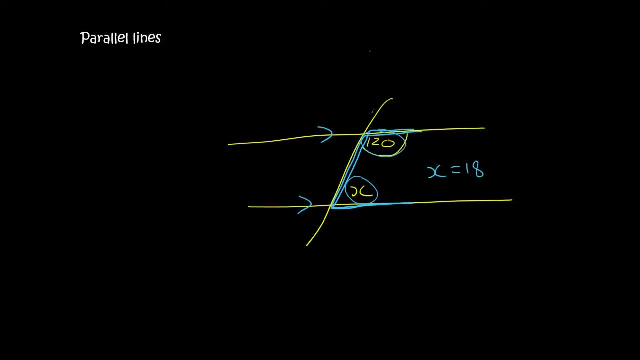 not the same, but they do add up to 180, so x would equal to 180 minus 120, and so x will be 60 degrees. i want to know how much is, or how much this one is. so we need to look at the shape that they are. 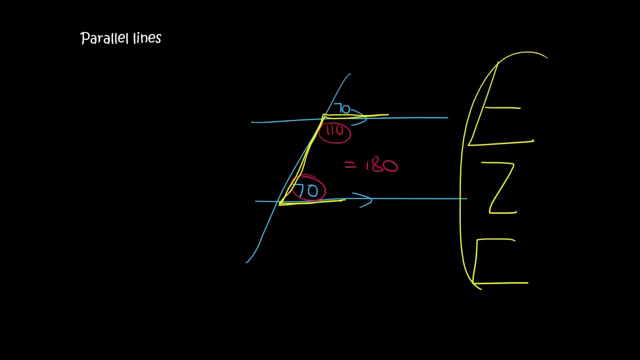 a u. so we've got something like that. so these are the types of shapes you need to look for. you need to look for a shape with an f, a shape with a u and a shape with a z or an n, and so always remember, when you're dealing with parallel lines, they are fun, okay? so if you can remember these three things, 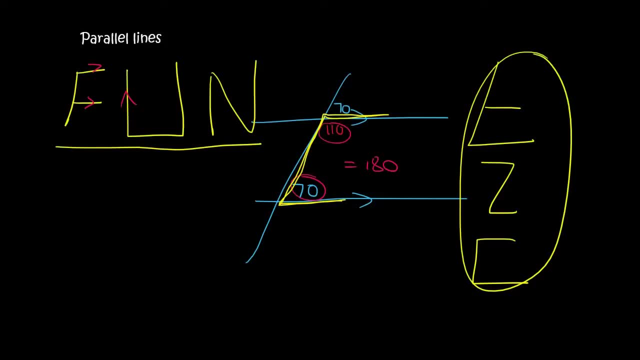 then you're good, so those lines over there would be parallel, those lines must be parallel, and those lines must be parallel. so then these angles are always equal. these two over here always add up to 180. they are not equal, but then these ones are always going to be equal to each other. the f: 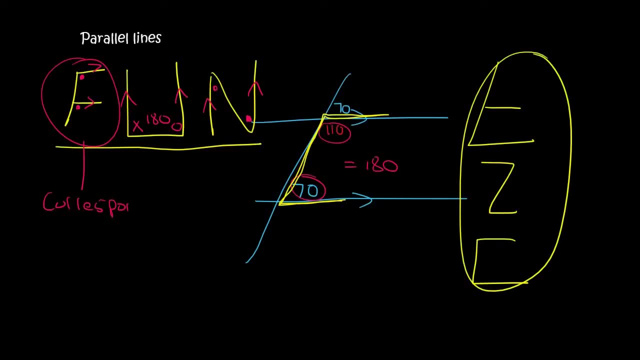 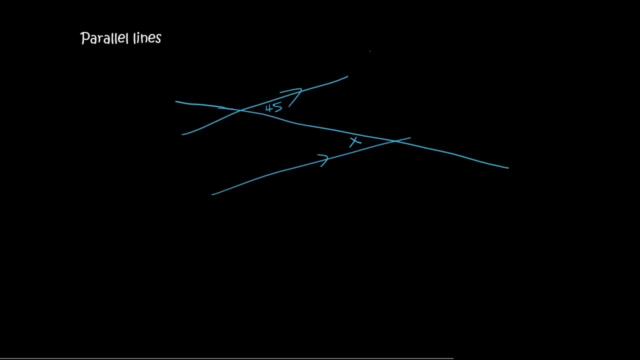 is called corresponding. in a test you can't say because of the f, but the f is called corresponding, the u is called co in teria and then the n or the z is called alternating. all right, so if i look at this diagram over here, i've got two parallel lines. how do i? 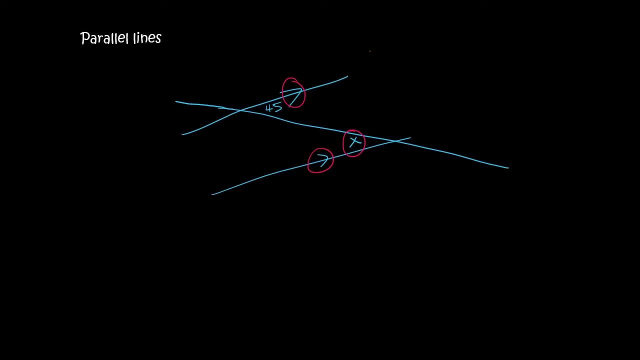 know that because of these arrows. i want to know what x is, and i want to know whether it's the u, the f or the z or the n. the z and the n can be the z can look like that, or it can be an n. oh, we can see that it's a z, so we know that angles in a z are the same, so x would equal. 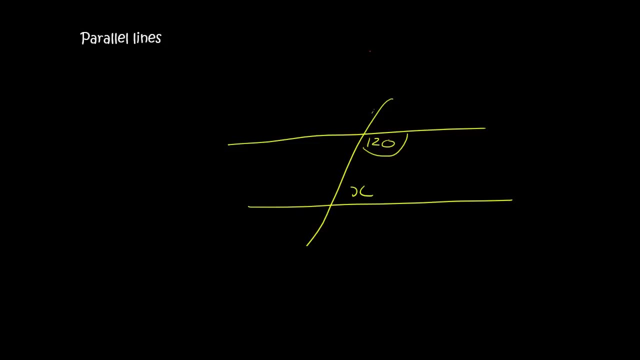 45.. if i look at this one now, this angle is 120. so what will this one be? well, the shape that these two are forming is the u, and remember, oh, and these two should be parallel. if you have a u, then they're not the same, but they do add up to 180, so x would equal to 180 minus 120, and so x will be 60 degrees. 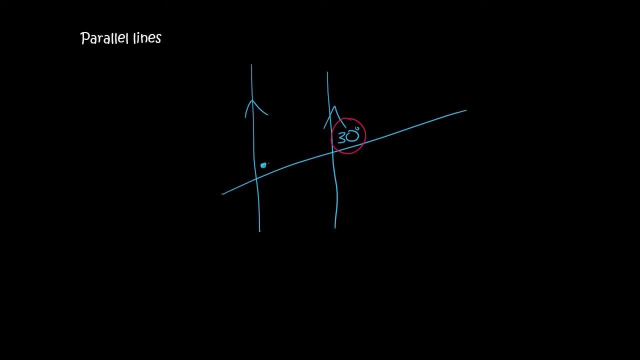 if you have a u, then these two are parallel, and so x will equal to 180, so x will equal to 180.. this one is so we need to look at the shape that they are forming. so if we do this there, we've got our f, and so this angle for the f stay the same, so this will also be 30 degrees, and 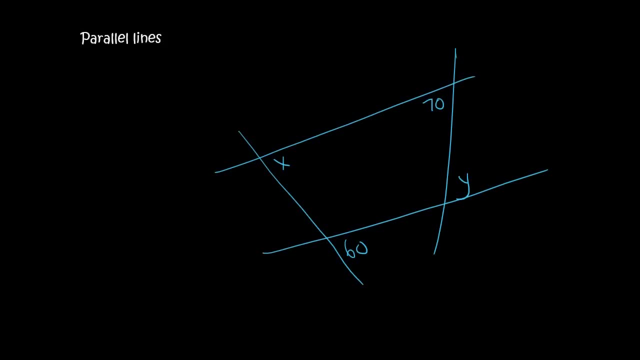 that's because of the f. all right, so here's, we're going to look for x and for y. oh, i must say that these lines are parallel, okay. so if we look at the x and the 60, well, that shape is an f, so x would be. 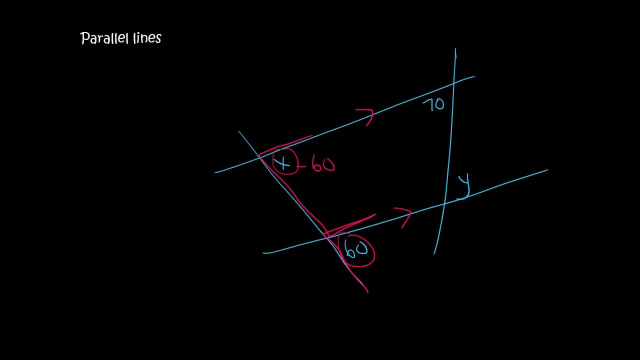 60. I'm not worrying about the reasons just yet, I'm just getting you guys into the hang of this, or into the swing of things. if I look at the 70 and the y and I form the shape, that's a z, so y would be 70, okay. so here we need to find x, y and z. so for the x one we can see that this shape. 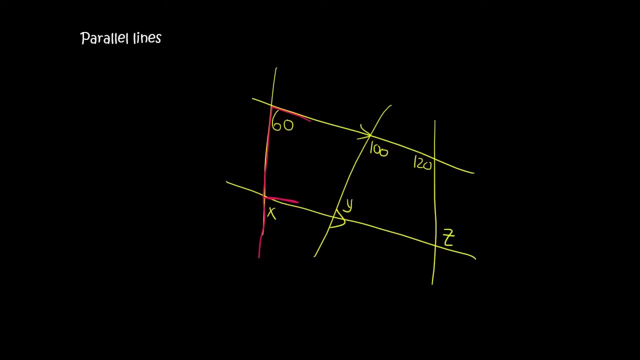 here is a f, so x would be 60. if we look at the next one, the y and the hundred, well, that shape, there is a u. so remember, with a u they don't add up, I mean they don't equal each other, but they rather add up to 180. so this one would have to be 80 degrees. and then, if we look at the last one, 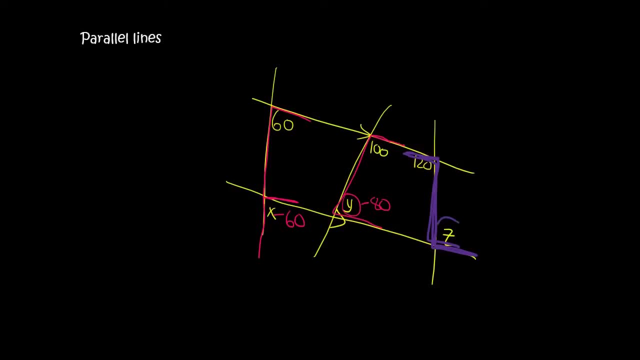 we've got a z and so the z's are equal, so this is 120.. Okay, So here's another one. so with the 70 and the x, if we form the shape, that's a z. it's a bit of a backward z, but it is a z shape as long as it does something like this or like this, like that, like. 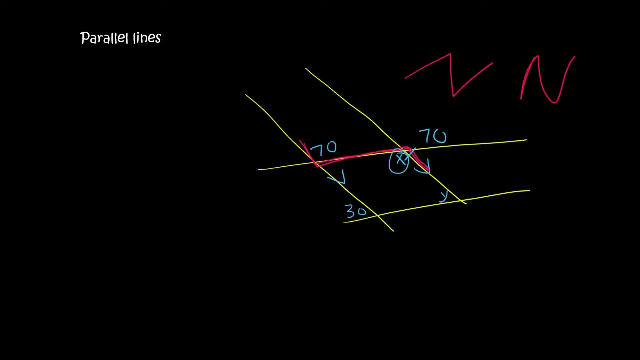 that it doesn't matter. so that means the x will be 70 degrees. if I look at the shape that is being formed over here, that is an f, and so y will be 30 degrees, and here's the last one. so if we look at the 30 and the x, 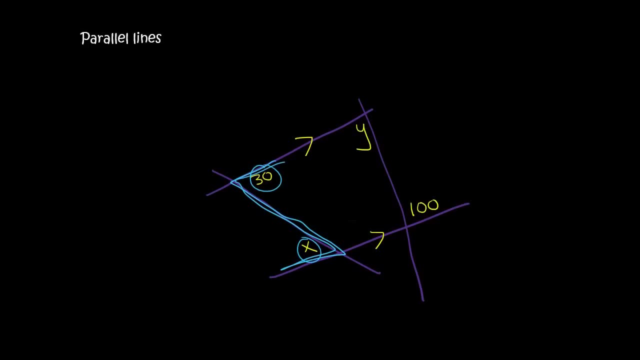 that is a z, and so x is 30. if I look at the y and the 100, ah, that's also a z, and so y is 100. and so there we have it, guys. a small little introduction to parallel lines. if you have parallel lines, please remember the f's, the u's and the n's.